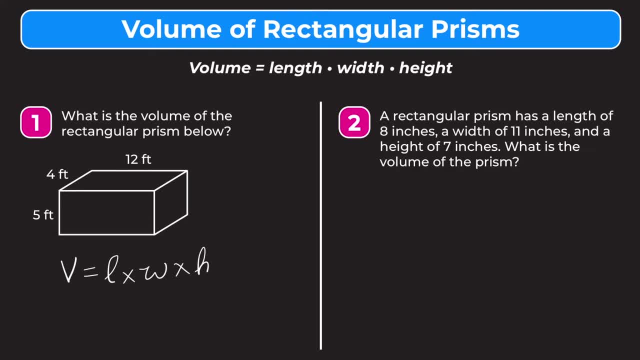 It doesn't matter which one we choose for our length and our width. our answer is going to be the same. So I usually choose the longer side for length. that's just me. but again, it doesn't really matter. So let's rewrite this: we have V equals, so our longer side for me would be 12, that would. 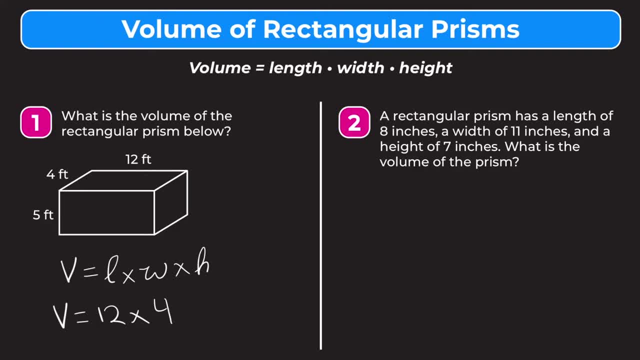 be our length. Our width then would be 4, so 12 times 4 and our height would be 5.. So let's go ahead and multiply these together, So we have our volume. I like to separate it out and do two numbers first and then multiply. 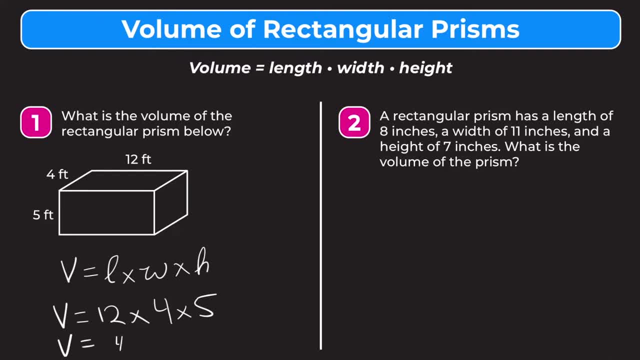 the last one. So I would do 12 times 4, that's going to be 48 times 5, and 48 times 5 equals 240.. So our answer here, for example 1, the volume of this rectangular prism is 240 feet. 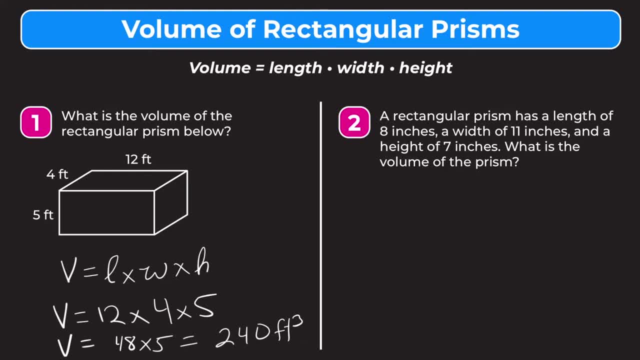 cubed. Your answer is always going to be in feet, in cubed feet. so feet cubed would be the unit of measure for your answer. So we circle that. Let's try number 2.. So for number 2, we don't have a rectangular prism drawn out. You can. 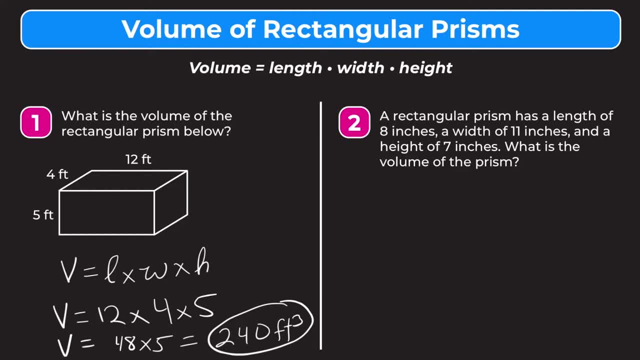 draw it out if it helps you. but if you realize, they give you the numbers for length and width and height written out, So you can just put those straight in there. So let's get into the formula. So again, if we write our formula, we have v equals length. 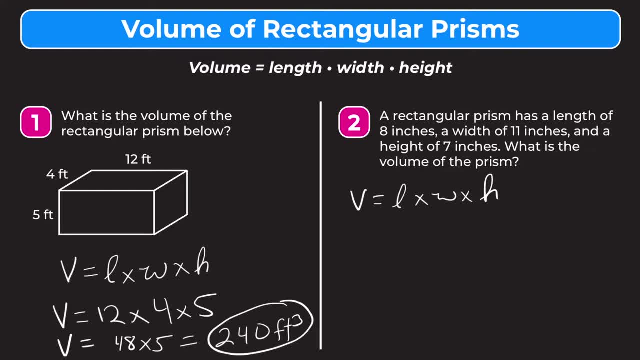 times width, times height. So now let's sub in our values. So it says in the problem: this prism has a length of 8, so 8 inches times a width of 11 inches and a height of 7 inches. So again, if we multiply this through, I like to do the first two first. 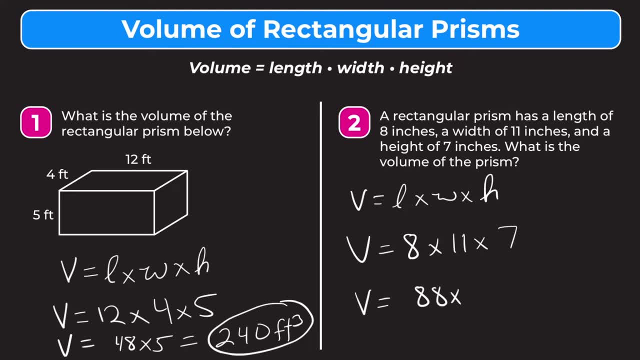 So 8 times 11 is 88, times 7, and then 88 times 7 equals 616.. And again that is going to be. in this example we have inches, not feet, so that's going to be 616 inches cubed. 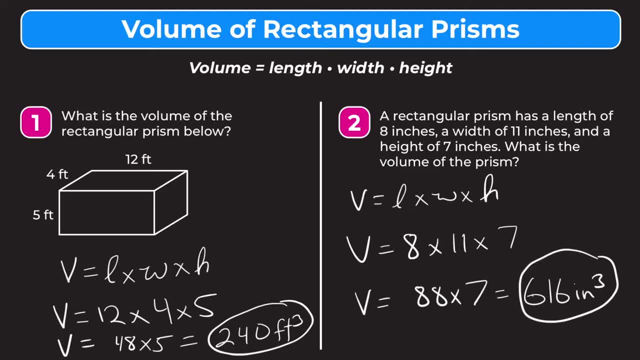 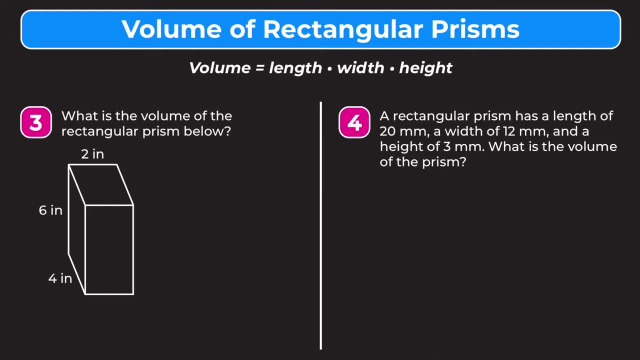 or 616 cubic inches. So if you have any problems, you can feel free to pause the video and try them on your own. if you're feeling confident Or if not, and you just want to follow along with me, that's fine as well. 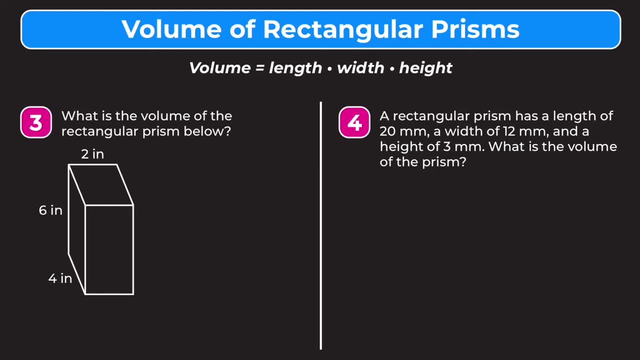 So for number 3, we have a rectangular prism drawn out here with the dimensions of 4 inches, 6 inches and 2 inches. So let's start by writing our formula. We have v equals l times w times h. Now let's 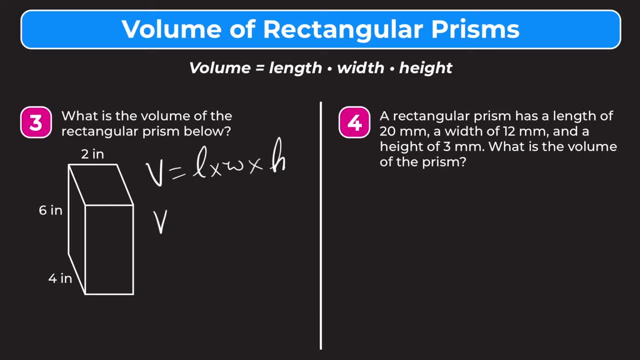 plug in our values, So v equals length. I always use a larger number, so we're going to say 4 for our length, times 2 for our width and then times 6 for our height. So now let's multiply these through: v equals 4 times 2 is 8, times 6, and 8 times 6 equals. 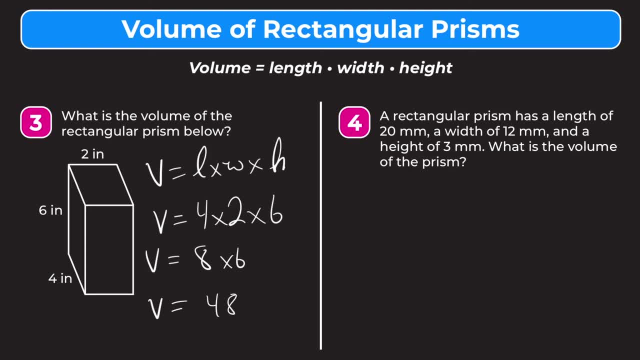 48.. And then remember, our unit of measure is inches, cubed or cubic inches. So our answer is 48 cubic inches. Let's try number 4.. This says a rectangular prism has a length of 20 millimeters, a width of 12 millimeters. 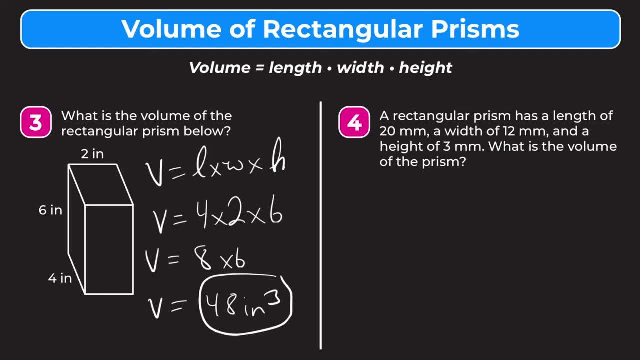 and a height of 3 millimeters, What is the volume of the prism? So we write out our formula: v equals length times width, times height. And now we plug in our numbers. The length the problem tells us is 20.. 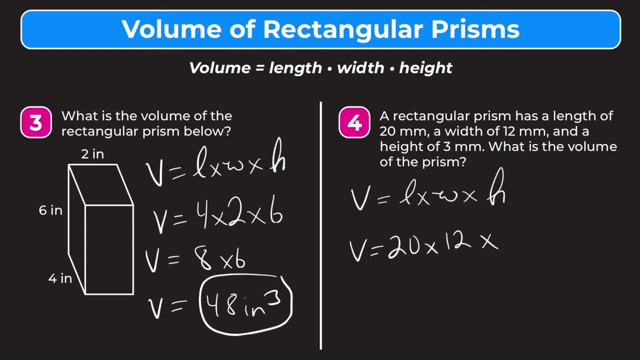 The width is 12. And the height is 3.. So now, if we multiply this out 20 times 12, is 240 times 3, and that is going to give us 720.. And our unit of measure is millimeters. 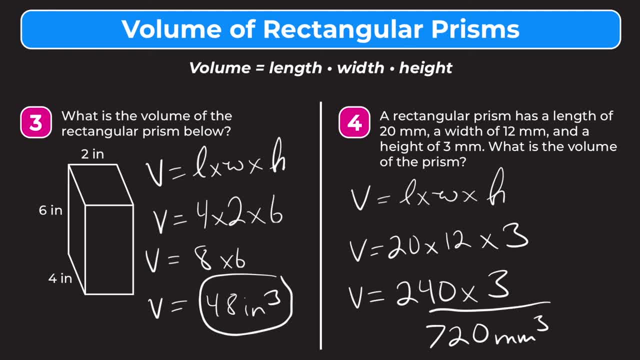 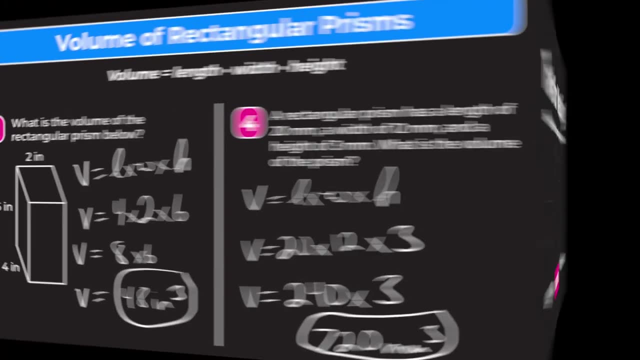 Millimeters cubed or 720 cubic millimeters. So hopefully, after watching this video, you all have a better understanding of how to find the volume of rectangular prisms. Thanks for watching and have a great rest of your day.